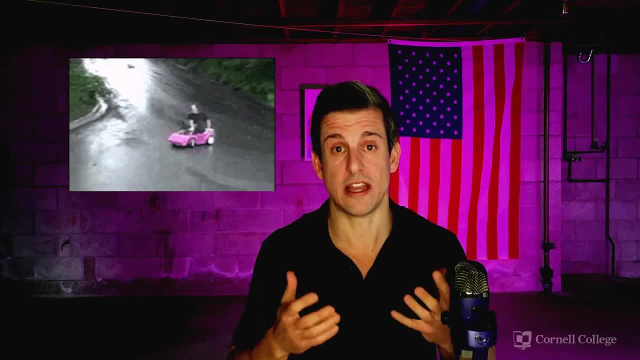 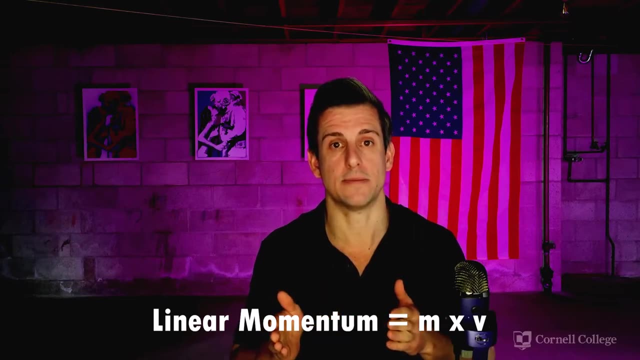 If your car is rolling down a hill, we say it has a lot of momentum. And why is that? Well, linear momentum is the mass times, the velocity. Okay. so the more mass something has and the faster it's moving, the more momentum it has. 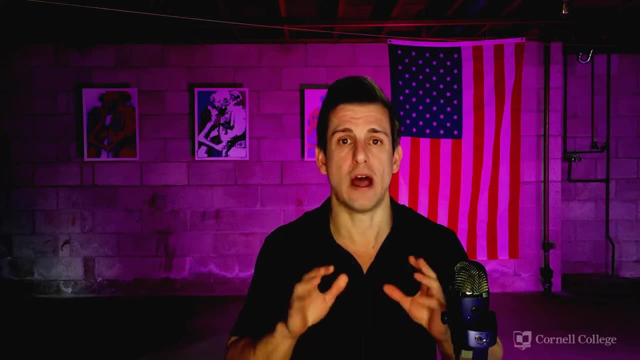 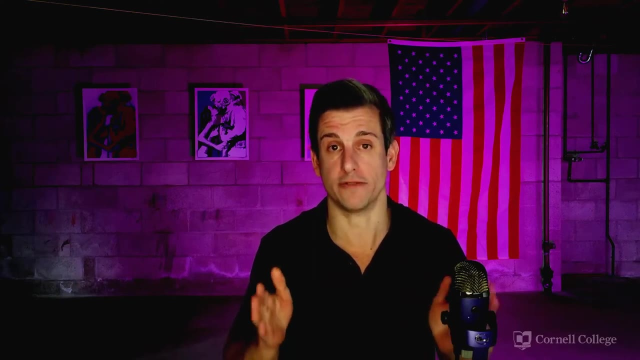 I think impulse is a little more trickier and maybe you haven't heard of an impulse before. A linear impulse is just a force acting for a specific amount of time. Okay, so let's do a quick example showing the relationship between momentum and impulse. 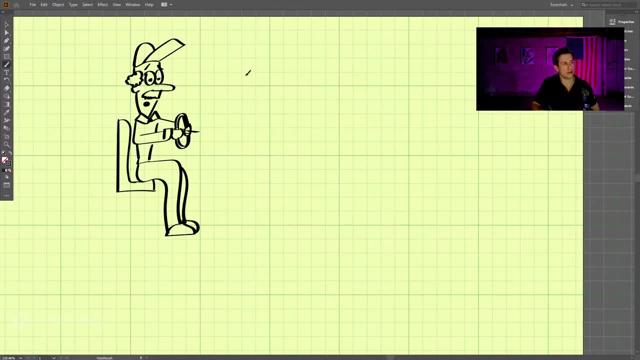 Okay, so we have this person in this car that's driving 30 miles per hour, And 30 miles per hour is also 13 meters per second. Now they unfortunately get into an accident and their head hits the steering wheel and comes to a complete stop. 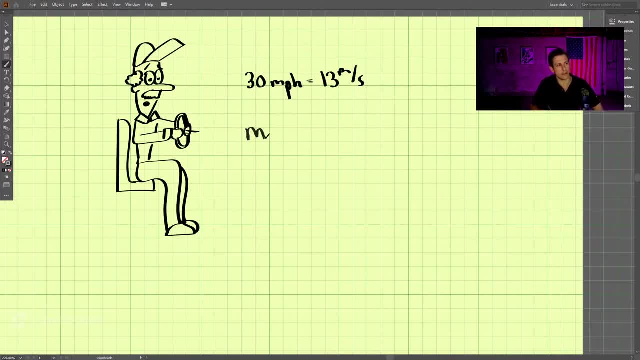 Okay, so what we have here, the equation that we use, is mv1 plus some constant force. We're going to assume that the force is constant over a certain amount of time. delta t equals mv2.. Okay, So in this case we consider mv1 and mv2 being measures of momentum. 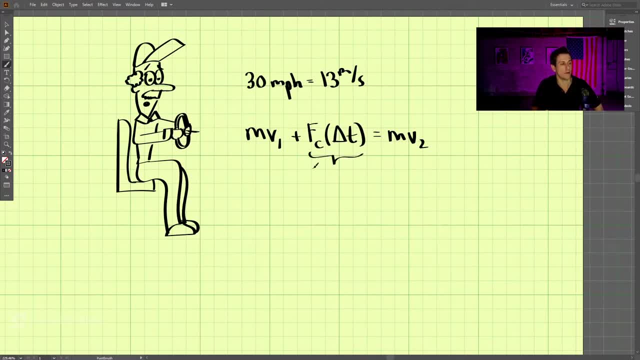 And this part right in here is the impulse. We call this the linear impulse. Well, if I spell it correctly, impulse. Okay, And so what is happening here? Let's assume that the person's head hits the steering wheel and the head has a mass of 5 kilograms. 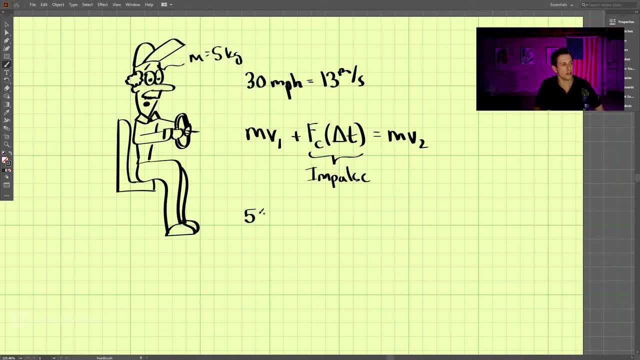 Okay. so if we do this calculation on the left-hand side, we have 5 kilograms times its initial velocity, which is 13 meters per second, plus fc times delta. t equals the mass times the velocity at state 2.. And we said it's going to come to a stop once it hits the steering wheel. so that is going to be zero on the right-hand side. 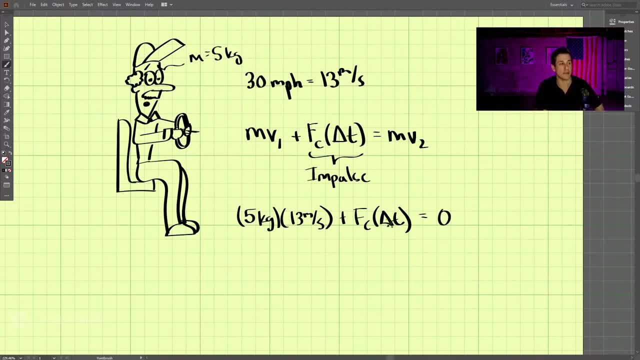 So we need to know what the amount, What the amount of time it takes to come to rest, And let's just assume that this is 5 milliseconds or 0.005 seconds. Okay, And that's just an approximation. Hitting the steering wheel, your head's going to stop pretty quickly. 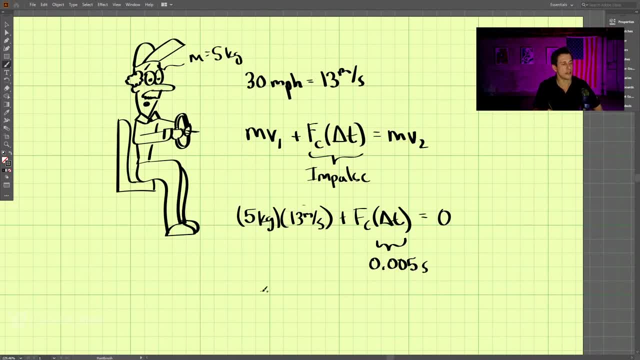 So let's just assume it's 5 milliseconds. Well, what we get here when we solve this equation is: fc comes out to be 13,000 newtons. Negative Negative 13,000 newtons. That means it's in the opposite direction of the head movement. 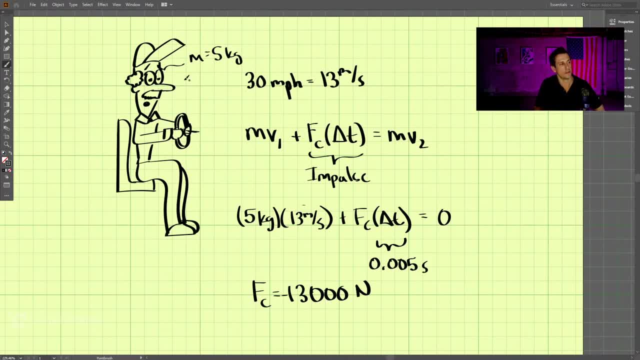 So if we consider the head being moved to the right here, the force applied by the steering wheel is back the other direction, So 13,000.. That's a lot of force. So to put that, to convert that that's almost 3,000 pounds. 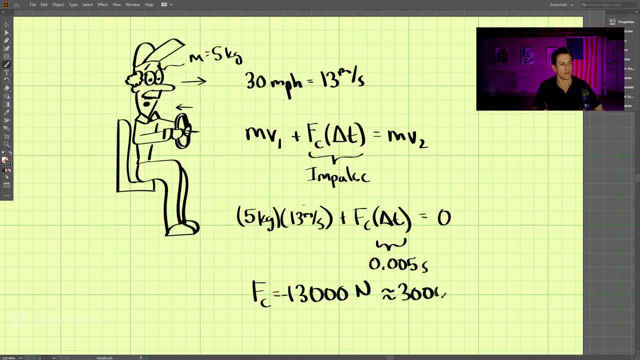 So approximately 3,000 pounds Being applied to the steering wheel- Probably enough to kill you. Okay, Now, since we have modern day cars, we've instrumented airbags into cars. So what is the airbag actually doing? 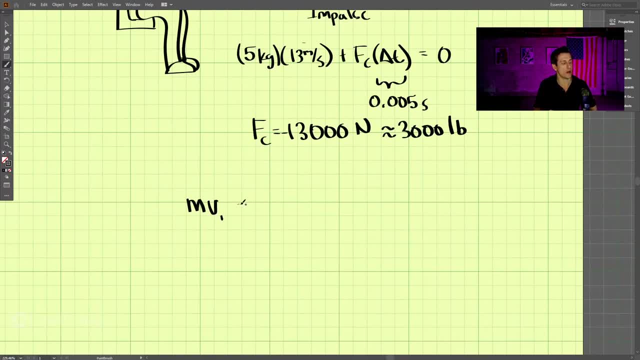 Well, let's take a look at this equation again. So we have mv1 plus some force times. delta t equals mv2.. Alright, The head is still coming to a stop with an airbag. Alright, Let's put that at 0.. 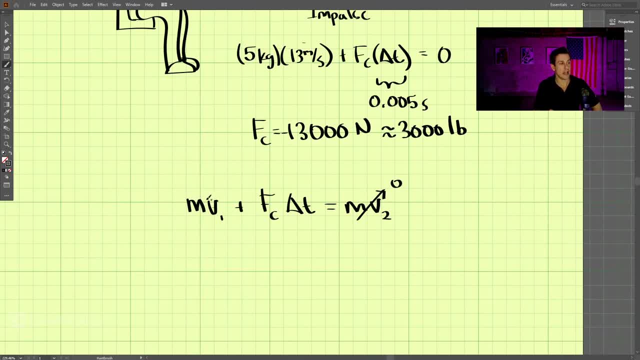 And the initial velocity and the mass is still the same, Right. So we have 5 times 13, still, Alright. So if we write out this equation, alright, the amount of time that the head comes in contact with an airbag is much longer. 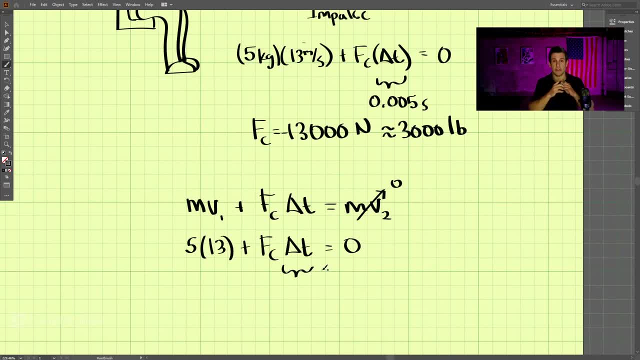 Right, That's what it's doing, Right. The airbag inflates, Your head hits it, It squishes in the airbag as it goes in. So this is actually the time your head is in contact with an airbag is about 80 milliseconds. 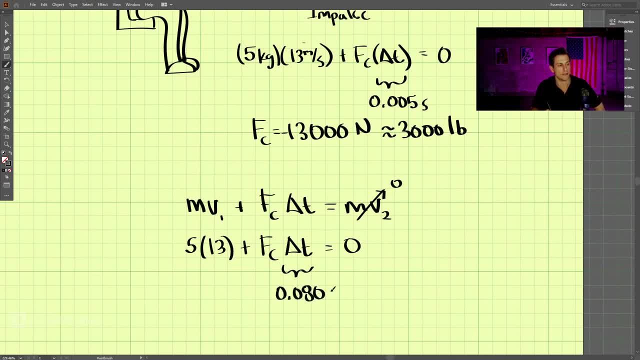 So that's 0.080 seconds, Alright. So if we perform this calculation again, let's perform that quickly. FC comes out to be negative 812.5 newtons, Alright, And that is roughly Equivalent to 190 pounds. Right. So people that have been in accidents where an airbag's been deployed: they still say that it hurts like getting punched in the face. Right, 190 pounds would feel like getting punched in the face But at the same time, right, it's much better than 3,000 pounds if your head comes in contact with the steering wheel.